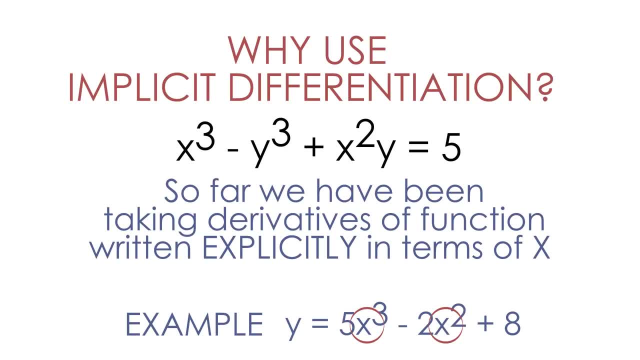 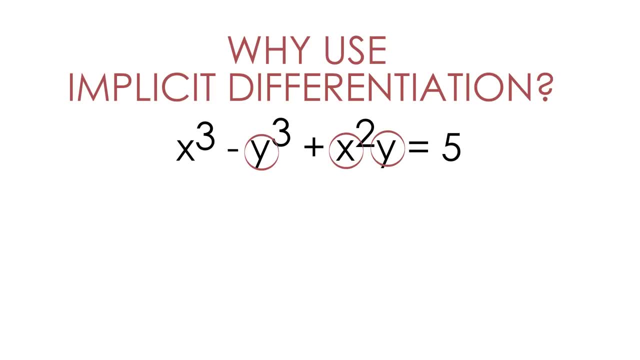 In terms of x, so we can use standard differentiation. But in this example, notice how we have x terms and y terms that are combined together, So they are not written explicitly in terms of x. So we must use implicit differentiation to find the derivative. But don't worry, using implicit. 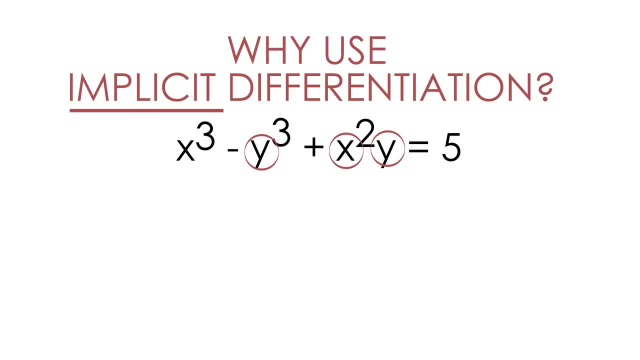 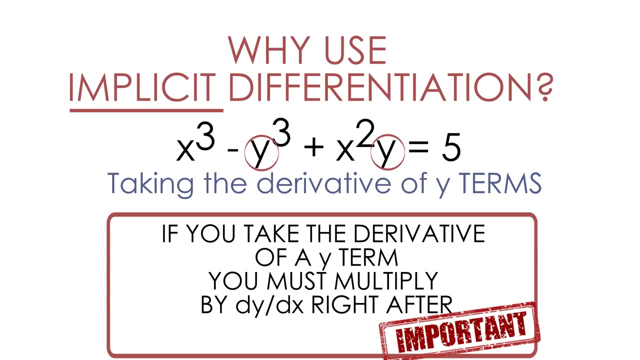 differentiation is not much different than what we've been doing already. The main difference is that we'll be taking the derivative of y terms, And the one thing that you have to remember is, if you take the derivative of a y term, you must multiply dy, dx right after that term, And you'll see what I mean by this once we 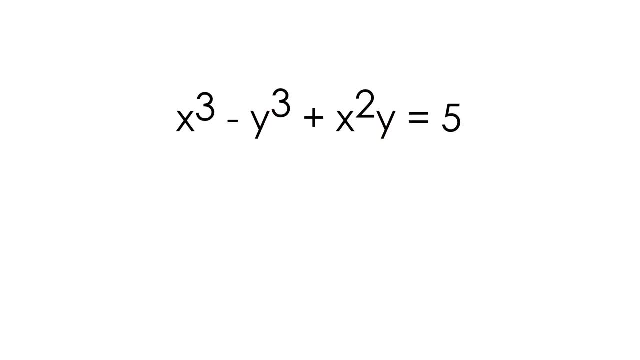 get started with this example. So let's get started right away. So let's start on the left hand side of our equation and take the derivative of our x cubed term. The first thing we do is take our exponent of 3 and multiply it in front. 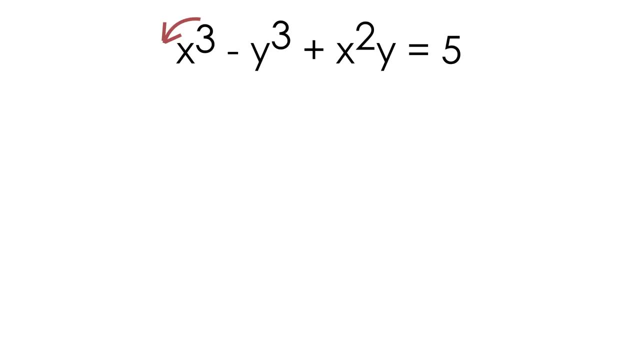 of the x. So the new exponent is going to be subtracted by 1.. 3 minus 1 is equal to 2.. All right, So now let's move a little bit to the right and take the derivative of the negative. 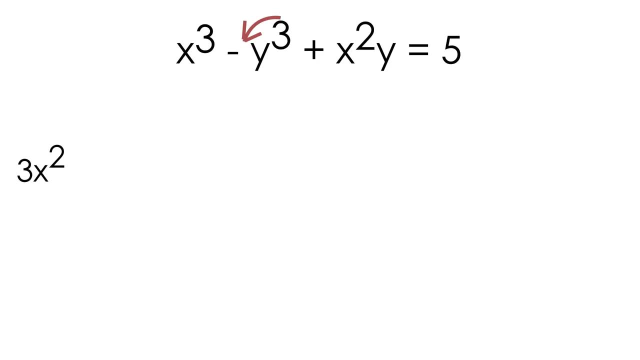 y cubed. Once again, we'll take our exponent of 3 and move it to the front of the y term. Our new exponent will be subtracted by 1.. So 3 minus 1 is equal to 2.. And remember what I said earlier: We must multiply. 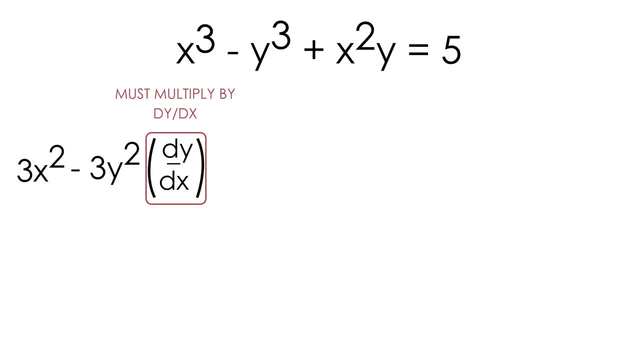 the derivative of a y term. So let's multiply this by dy, dx. All right, so now let's keep moving to the right and let's take the derivative of our x squared y term And notice that we have two things being multiplied with each other. We have the x squared being multiplied with the y, And whenever 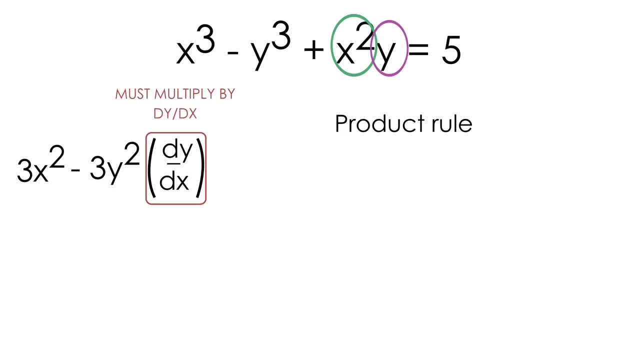 you have two things being multiplied with each other. we have to use the product rule to take the derivative, And what I like to do when using the product rule is to label our first term, which is x, squared the first, and to label the second term, y, the second, And the formula for. 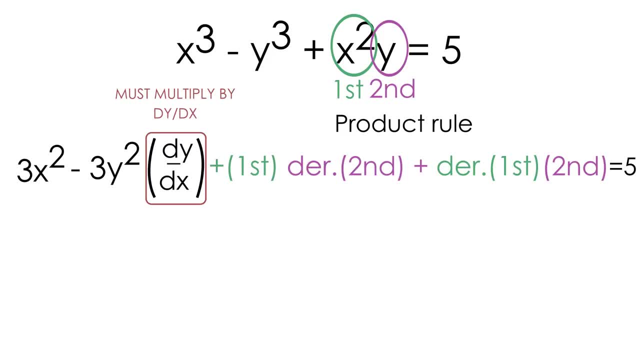 the product rule is the first term times the derivative of the second term plus the derivative of the first term multiplied by the second term. All right, so let's plug in our first term of x- squared every time we see the word first- And let's plug in our second term of y. 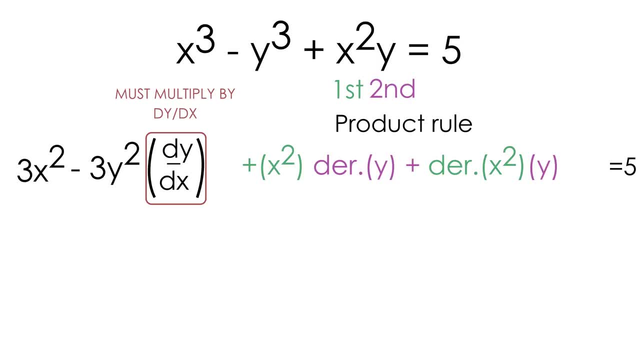 every time we see the word second. All right, so now let's simplify this product rule portion of our problem and take the derivative of y. Now the derivative of y is just equal to one And once again we took the derivative of a y term. so we must multiply this by dy dx. 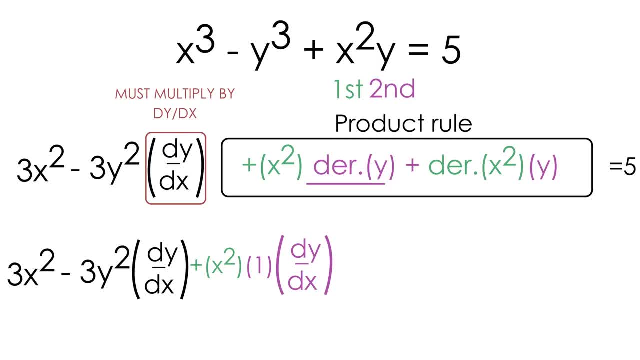 And if we keep moving to the right now, we can take the derivative of our x squared term. The derivative of x squared is equal to 2x, All right, so now, at this point, we can keep moving to the right and take the derivative of our constant of 5 on the right-hand side of the. 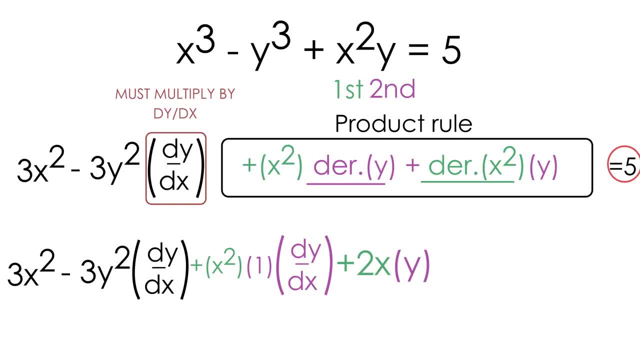 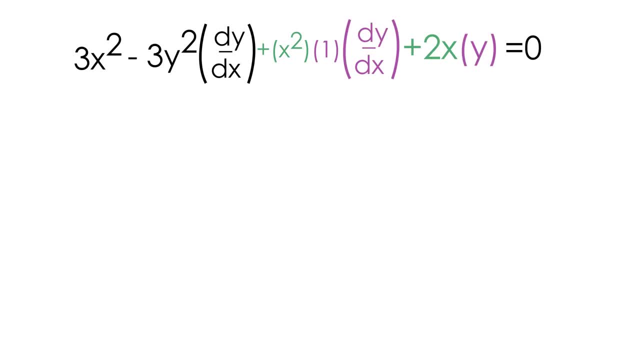 equation, And we know that the derivative of any constant is equal to 0.. All right, so now that we took the derivative of every single term in our equation, the only thing we have left to do is solve for dy dx, And to do this just. 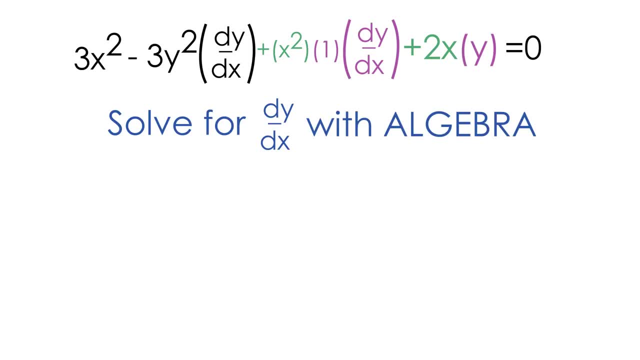 requires a little bit of algebra. The first thing I'll do is simplify the x squared times 1 times dx. x squared times 1 is just equal to x squared, and the dy dx stays the same. And we can also simplify the 2x times y: That is just equal to 2xy. All right, so once again. 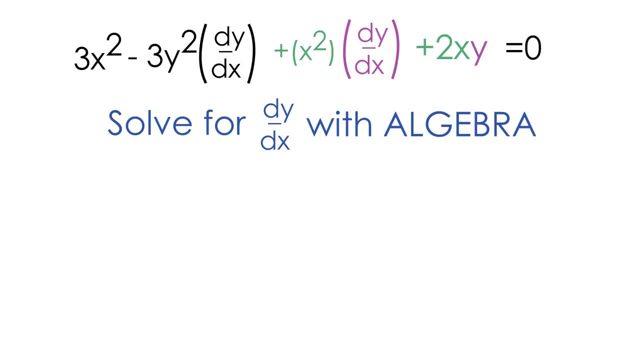 we need to solve for dy dx. So to do this, let's get all of our dy dx terms on one side of the equation and all of the other terms on the other side of the equation. So the 3x squared and the positive 2xy are both non-dy dx terms. Let's get them to the other side of the equation. 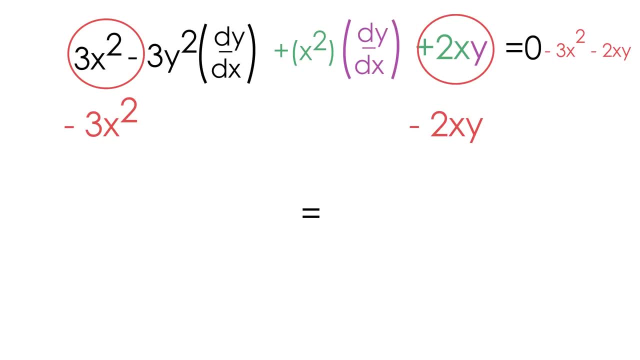 We can do this by subtracting 3x squared from both sides and by subtracting 2xy from both sides. And notice, on the left-hand side of the equation, the 3x squared and the negative 3x squared cancel each other out. The positive 2xy and the negative 2xy also cancel each other out, And the only thing.